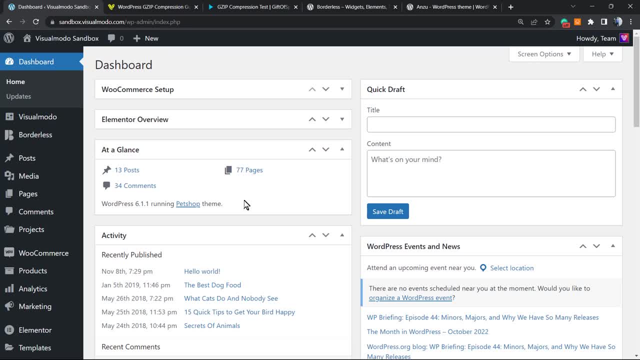 for WordPress dashboard. okay, I always like to start the videos on the dashboard to make it equal for everyone, and before we can continue, please take a moment to hit the subscribe button, like this video and share this content with a friend of yours. you have no idea how much it. 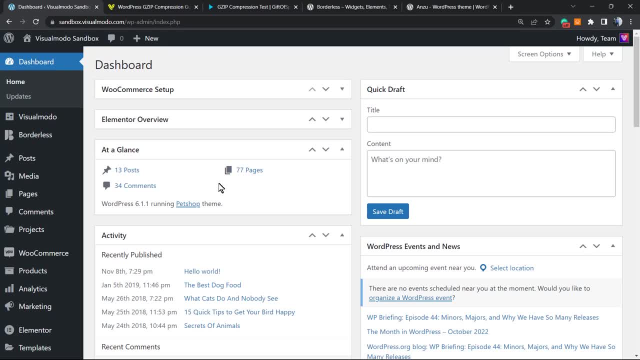 helped us because we bring daily videos about WordPress, SEO, plugins, technology and tools and everything you need in order to use internet on your site's favor. so let's get it started from the dashboard. review the left side of menu and you scroll it down until you can see the 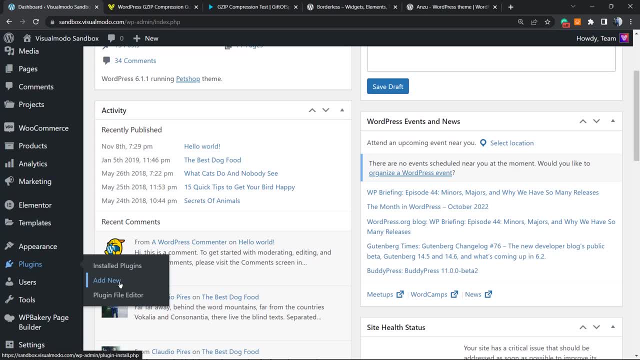 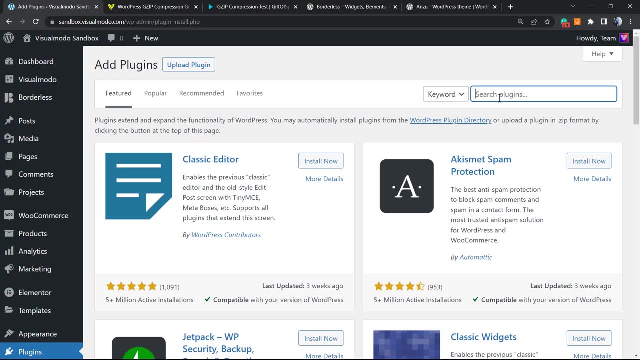 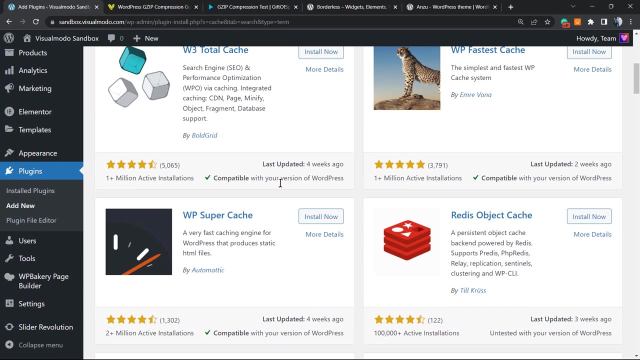 next menu, hover your mouse over it and click on add new. right here into the search plugins field at the upper right corner, we're gonna type cash, just like this. okay, scroll it down just a little bit and this is the guy that we're looking for. WP super catch. as you can see, it's activated into. 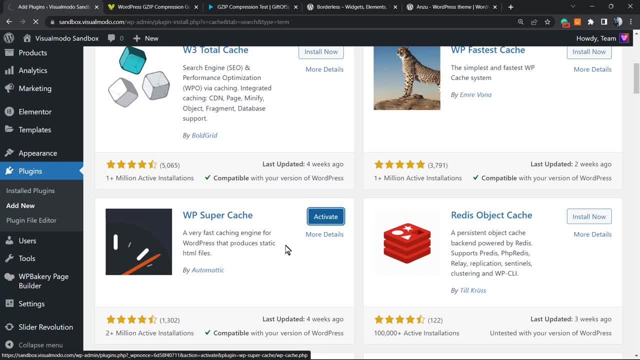 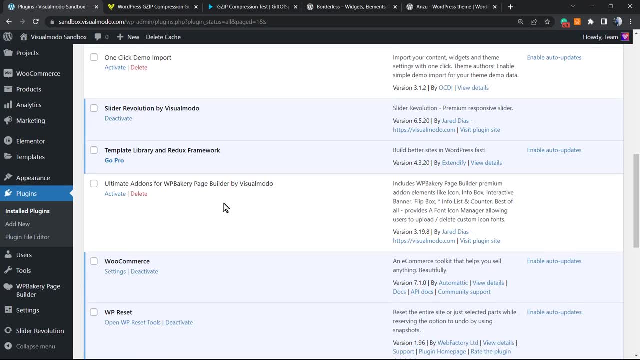 million websites. okay, so we're gonna click on install activated and it's gonna redirect us to the plugins list of our WordPress website. let's just screw it down so you can find the plugin. here is the WP super cash. we can access the settings from here, or 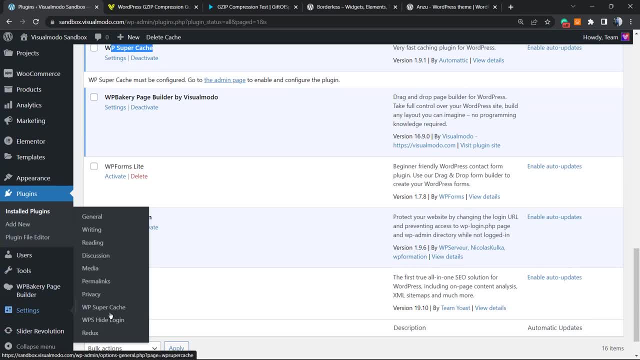 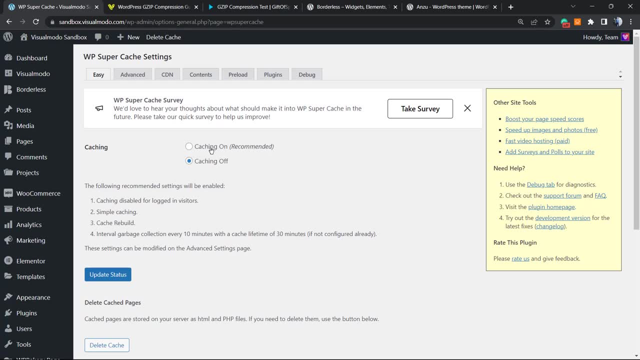 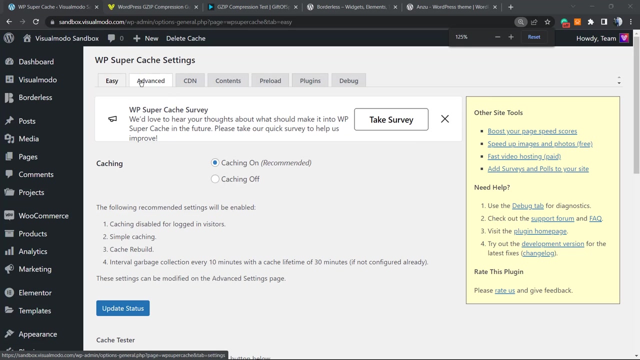 from the settings: left side menu, left sidebar menu and WP super cash. I'm gonna click on it. as you can see, the caching is off. I'm gonna set as on, as recommended. okay, let me update the status of updated. now I must go to the advanced tab. okay, next to the easy, I'm 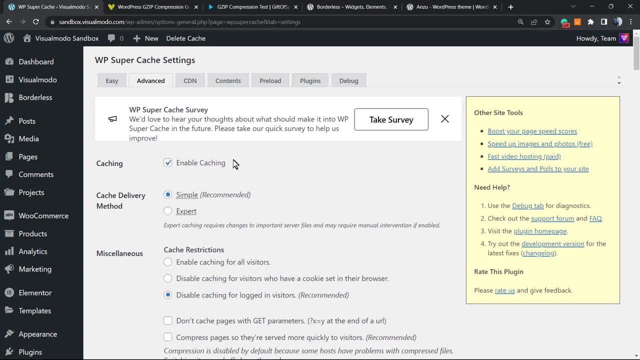 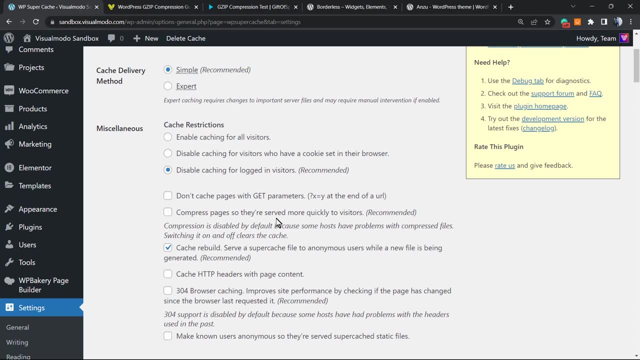 gonna move to advanced tab and from here all we have to do it's this simple: set compress page so they are servered more quickly to visitors. recommended compress is disabled by default because some hosts have problems with compressed files. switching it to on and off clears the cache. we're gonna click into this field right here. okay, this is very. 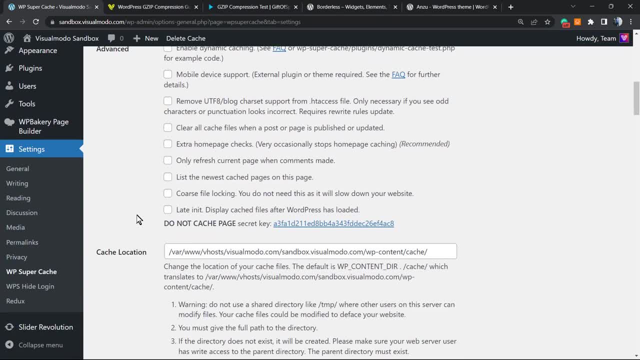 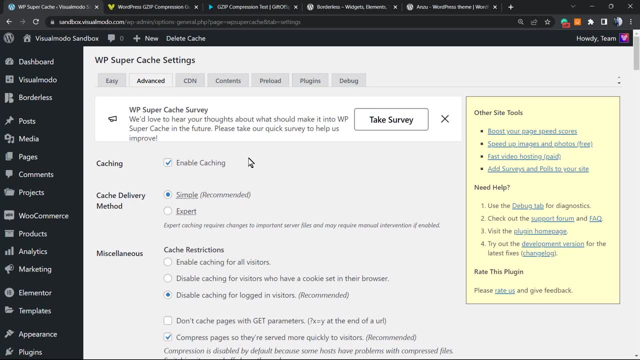 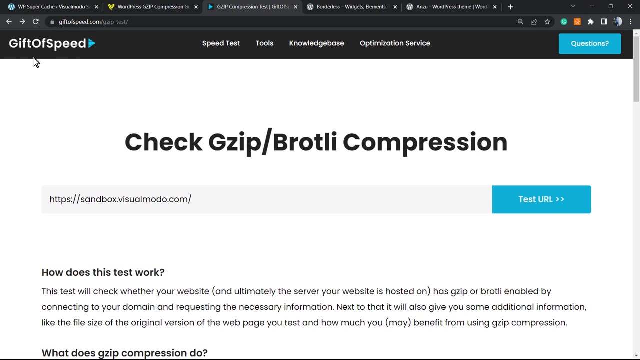 important. this is the whole point of the guide. click on it, scroll down, scroll down, scroll down and click on update status. okay, simple, easy and fast. okay, what else we have to do? let's check if it's working or not. here is the site gift of speed. you can do a lot of speed optimization. 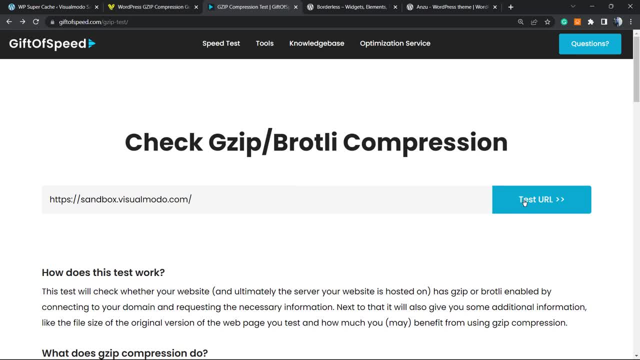 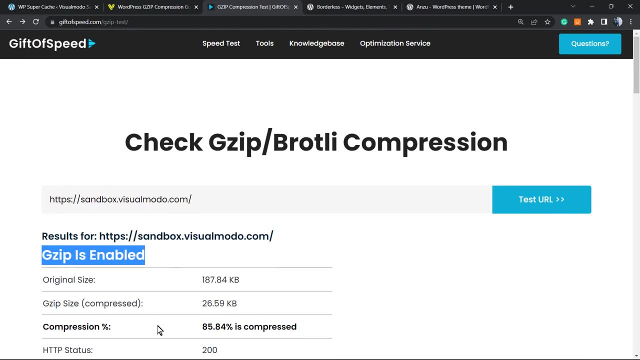 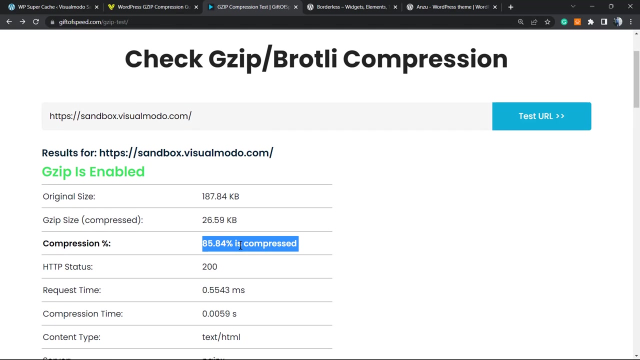 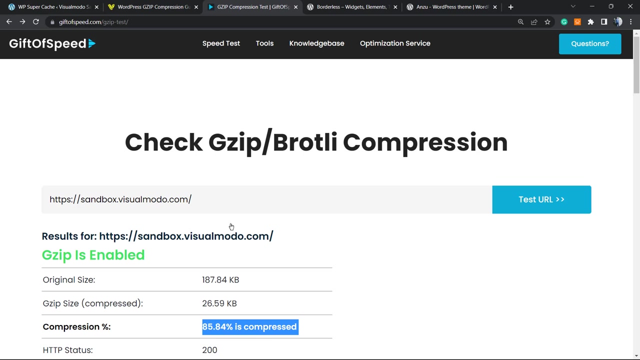 optimization checks on your site right here, click on test URL and gzip it's enabled okay. as you can see, it's up to 80 percent active. compress it okay, so it's a lot of compression level. this helps a lot the website optimization to speed and improve it. okay, and as you can check. 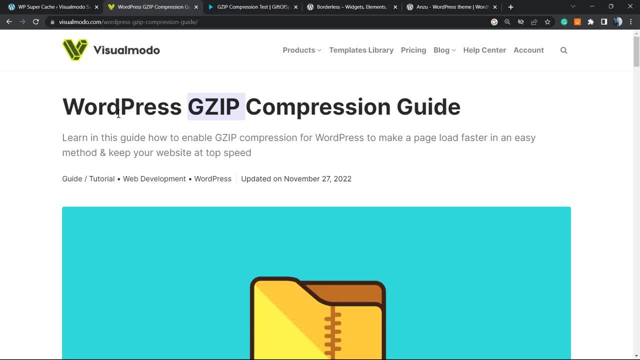 we have, we are capable to do this fast and for free, and that is. I hope you guys enjoyed this video. feel free to use the comment section below in the case that you have any question. don't forget to check out our borders. WordPress plugin in order to have more widgets elements. 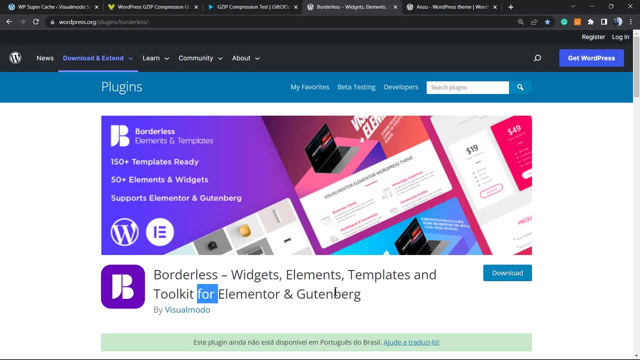 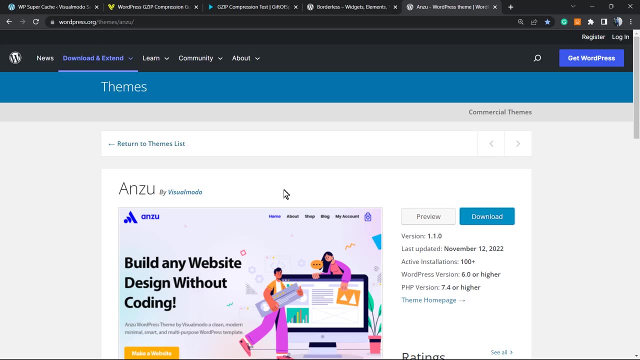 templates and tools for your WordPress page building experience, in order to have more pre-built websites that you can import for free with a single click. in addition, in the case that you are in needs of an amazing free WordPress team in order to have more templates, pre-built websites that you can import for free with a single click, 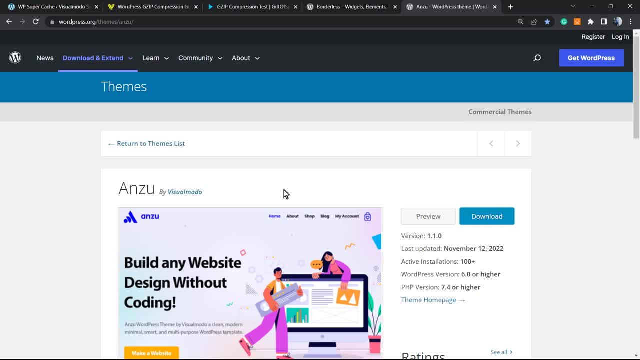 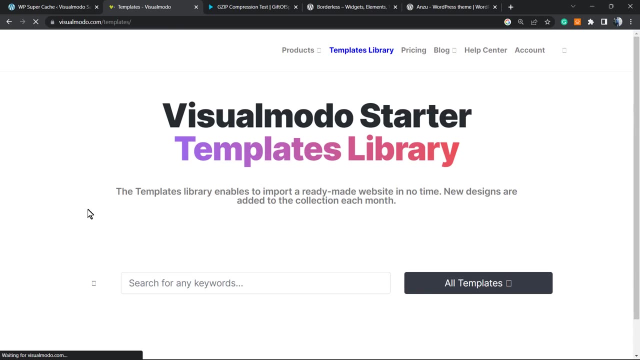 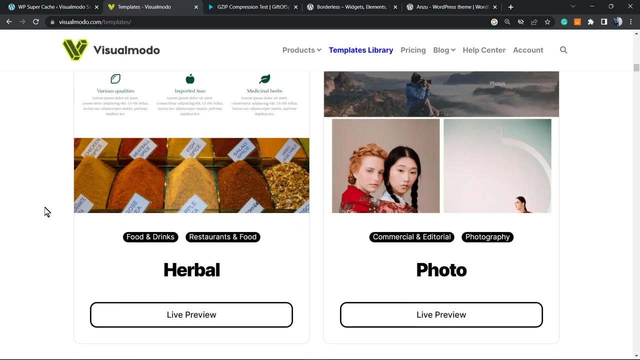 advanced menu search and other special widgets features: go to our WordPress dashboard appearance themes. add new search for Enzo. click on install and activate it completely for free. moreover, if you prefer to go premium and have complete support, premium icon packs, more pre-built websites, pages, plugins and extra design elements- go to visualmodocom. purchase the borders Pro or Enzo Pro licenses or. 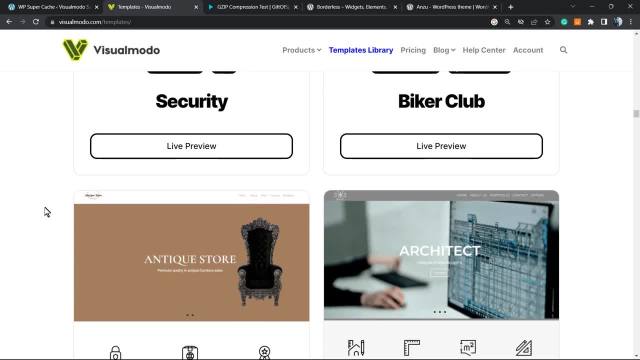 the visual motor plus that include both of their and it is. I hope you guys enjoy this video and I see you tomorrow. all the best.